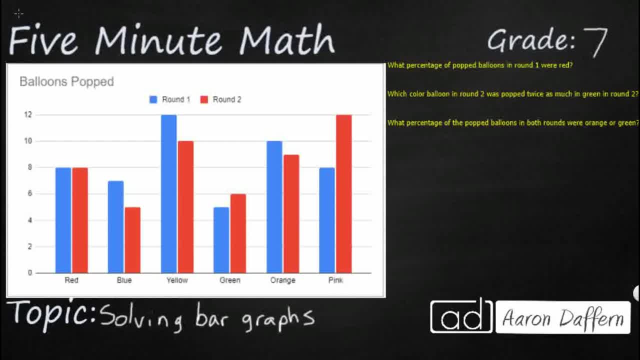 can do to make the bar graphs a little bit more complicated. Really, all that's going to happen is we are going to have different types of questions asked of us. So this is a basic bar graph here, and we have a scale interval of 2, and so let's just go ahead and do what we should. 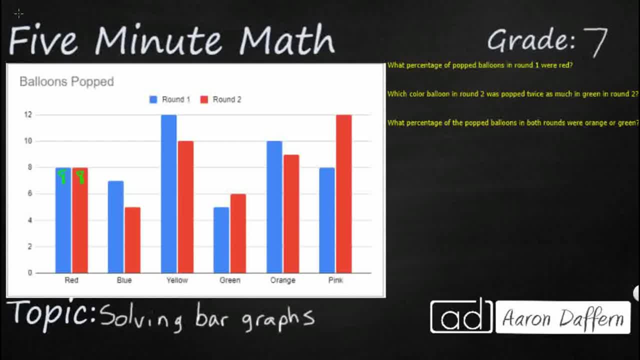 always do. Let's just put some numbers on. here We've got 8s, we've got some balloons that are popped apparently in two different rounds, so we've got 7 here and we've got 5 here. We'll need all these numbers in a moment. That's 12, 10.. Always, the best first thing to do is just go. 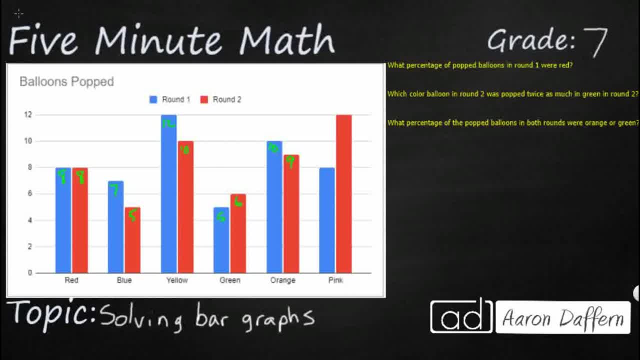 and put numbers on all of these, because you never know what you're going to need, and we are going to end up needing most, if not all of these. So let's look at our first question: What percentage of popped balloons in round 1 were red? 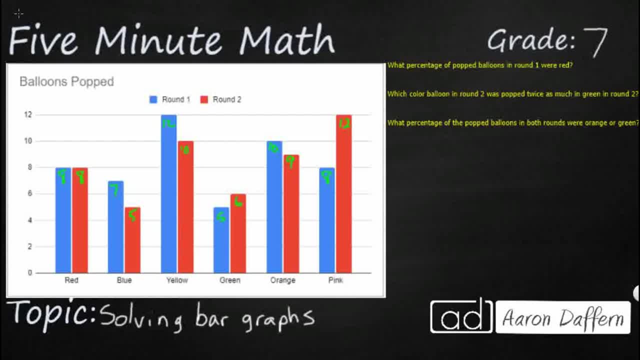 Well, let's deal with round 1.. So we need to first make a fraction, So we need to make red over all of round 1.. So first we need to make that fraction, Then we need to turn that fraction into a percent. 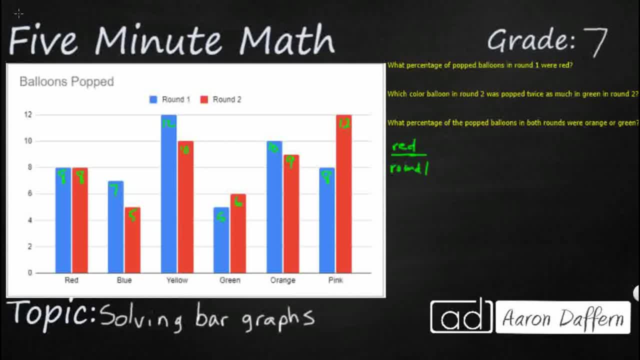 So how many red do we have in round 1?? Round 1 is the blue one, so it is going to be 8 over. now we've got to add up all of round 1, so that's why we went ahead and did that. So let me see. 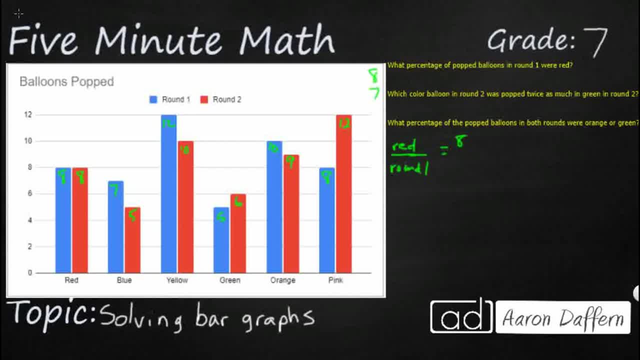 I've got 8,, 7,- just make sure I'm pulling the blue ones- 12,, 5,, 10, and 8.. Alright, so that's 10,, that's 12,, so that's 22,, that's 30. That's a nice, even 50. Alright, so 8 out of 50. So I have two options here. 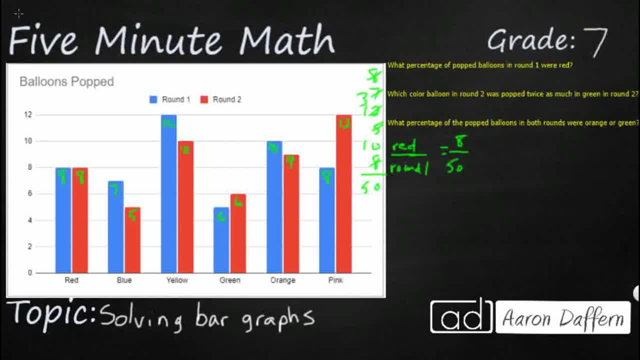 I want to change this into a percent 1,, to change it into a decimal. First I can just divide up 8 into 50, into 8, but you know what I know of a better way If I can get my denominator into 10,, 100, or 1000,. 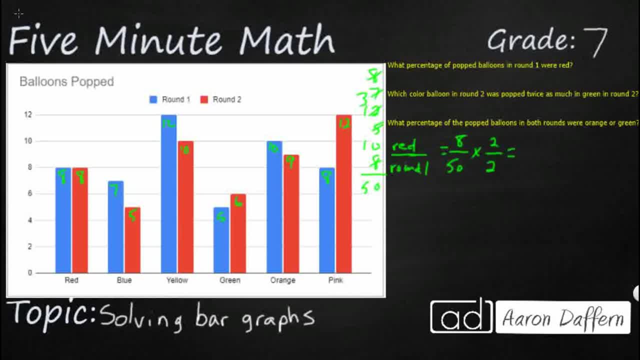 then it's going to be easy to turn it into a decimal, because those are the place values, the first three place values: 10s, 100s, 1000s. I see this 50, I know that if I double it I'm going to get 16 over 100,. 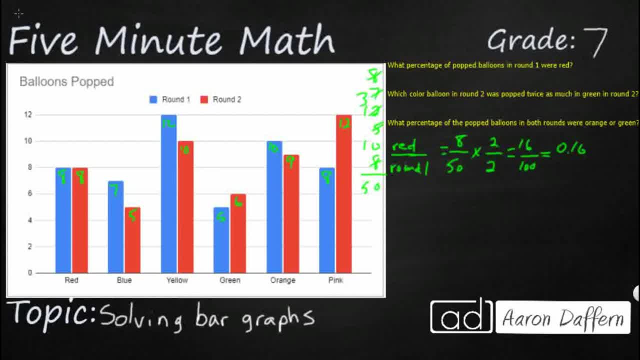 which is equal to 1600. Which is equal to move the decimal over twice: 1,, 2,, 16%. So there's my first answer right there. I've got 16% of the pop balloons in round 1 were red. Now which color balloon in round 2 was popped twice as much? 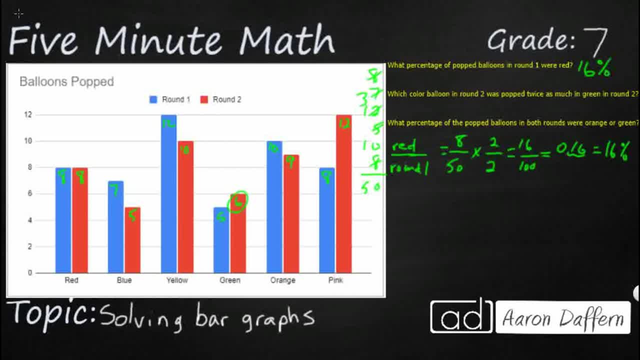 as green in round 2?? So green in round 2 is 6.. So twice as much as that. So I just need to double it. That's going to make 12. And I'm looking for round 2.. And there we go. I've got a pink right there. 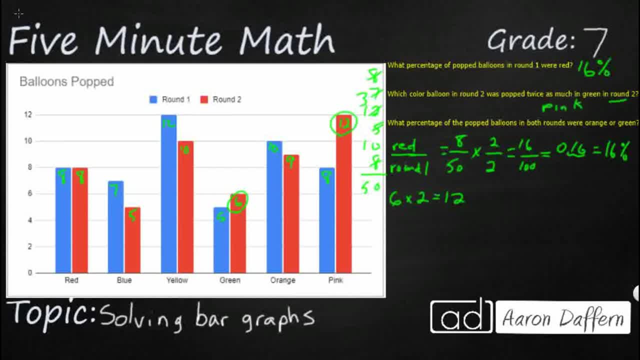 You might be thinking: oh, that's a simple problem. Well, it is. We just had to know that twice equals times 2. And it was easy because we already had all of our numbers. Let's check our last question here. 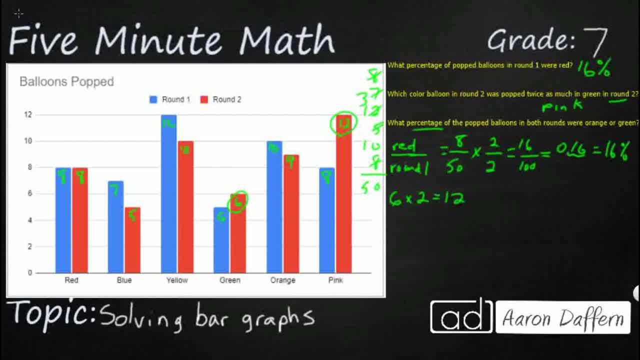 What percentage. so we're doing? another one of these of the pop balloons in both rounds were orange or green. All right, So I know how many balloons are in round 1, 50. I need to know how many balloons are in round 2.. 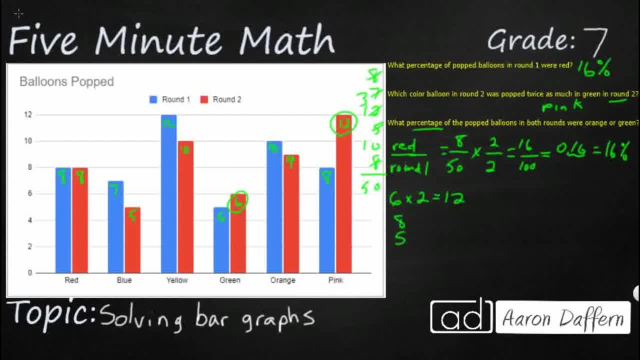 So let's just add that up here. I'm going to do 8,, 5,, 10,, 6,, 9, and 12.. So we add that up. Looking for 10s always, That's going to be 10.. That's 11.. That's 21.. That's 30.. Oh goodness. 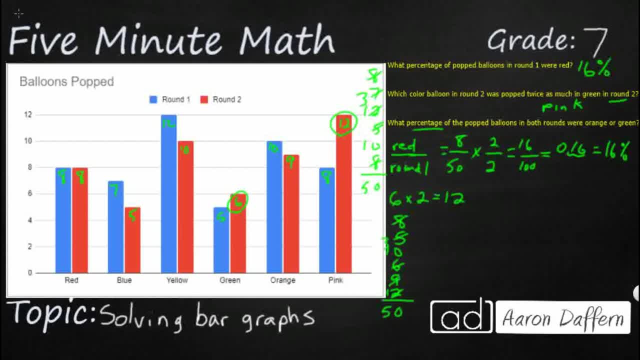 50 in each. So that's going to be easy because that's going to be over 100.. So I'm looking for orange or green, Orange or green, So I can get the sum of both of those And that's going to be over my total. That's round 1 and 2.. 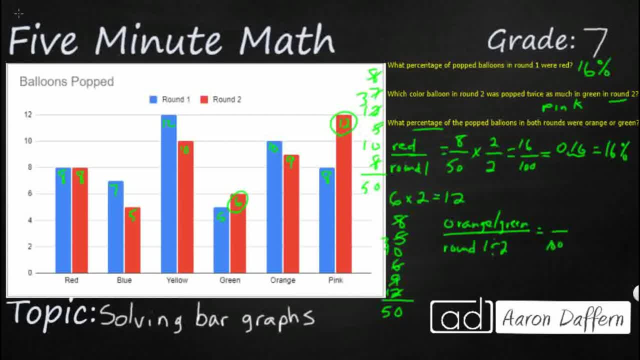 So that's going to be easy. That's 100, which is going to make a really easy percent. I need to get my total orange. I need to get my total green. So my oranges are 10 and 9.. Greens are going to be 5 and 6..